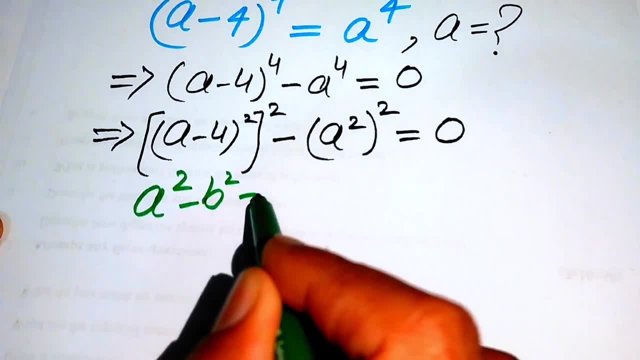 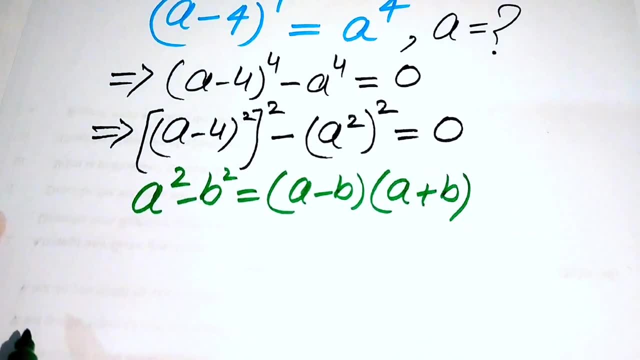 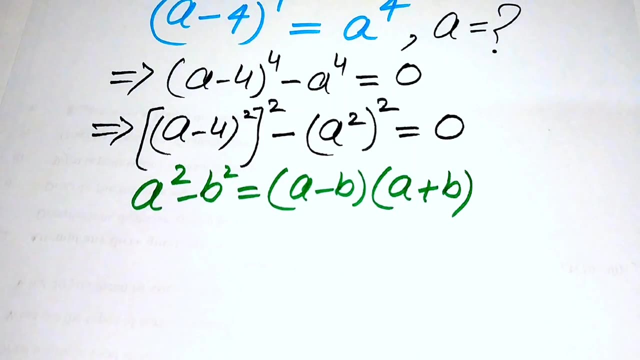 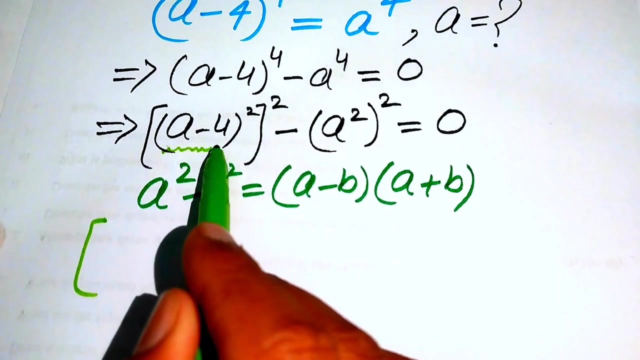 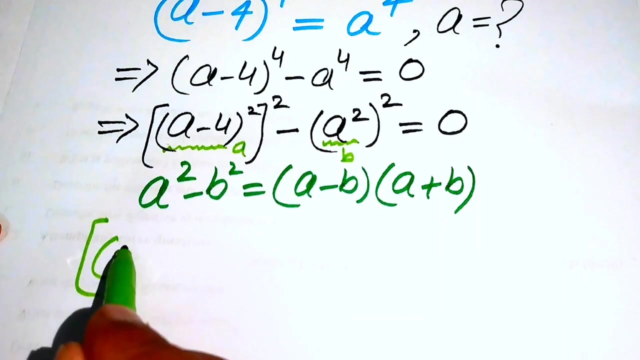 identity. if we have a square minus b square, it is equals to a minus b times of a plus b. so here we use this algebraic identity on the above term so that our above term will be written as in this form: so we have: this is the value of a and this is the value of b, so we have a minus b and we write it as a minus 4 square. 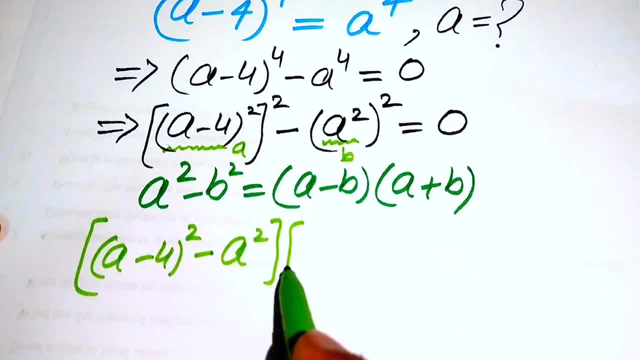 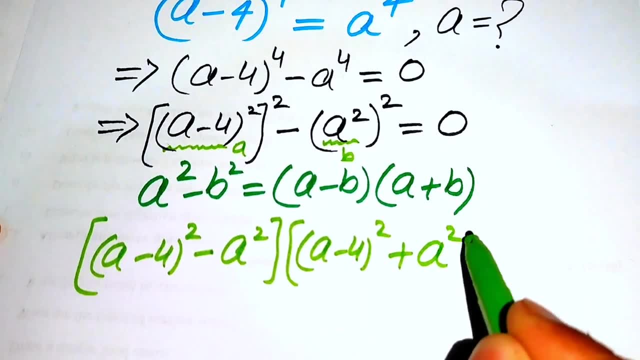 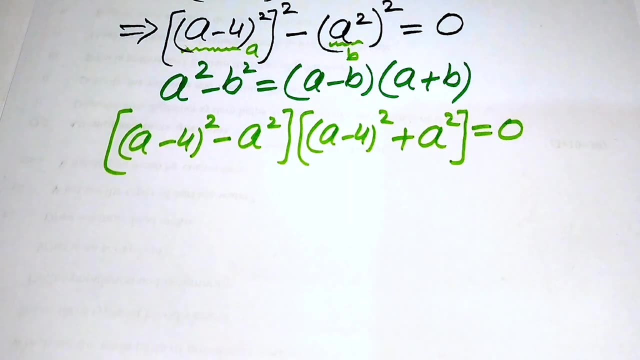 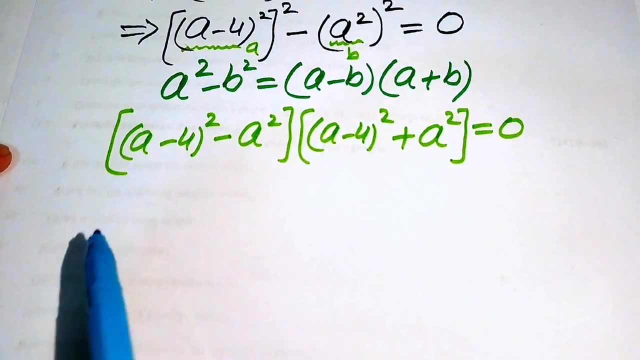 minus b is a square, into a plus b. so our a is a minus 4 square plus a square, and this whole equation equals to 0. and now, in the next step, we can just again use this algebraic identity on this term, and this term will be written as: 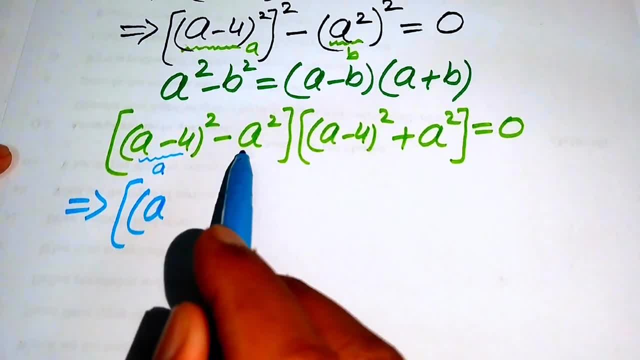 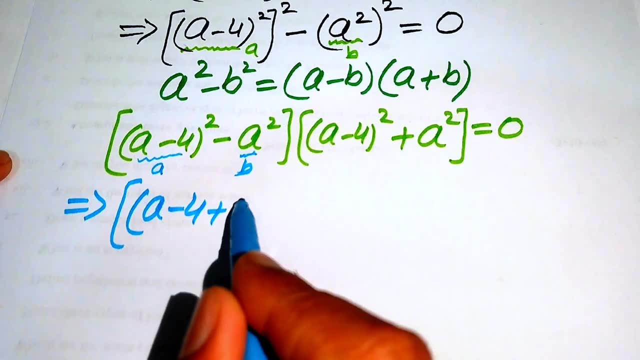 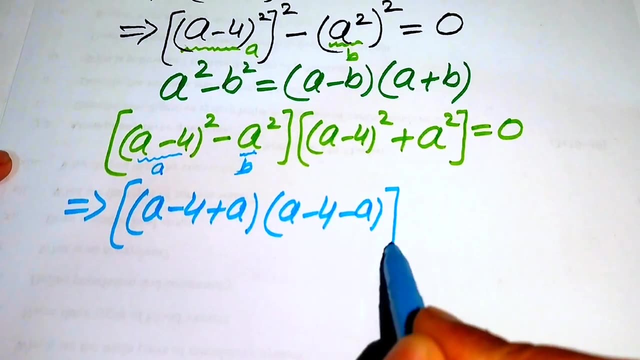 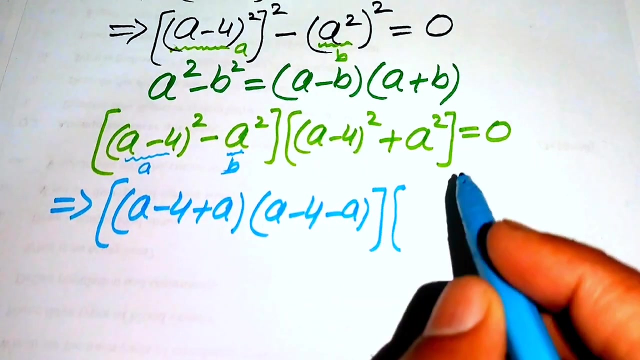 a square minus b square. so here, if we take this all term as a and this is b, so we again use this formula and we write it as a minus 4 plus a into a minus 4 minus a, and here we open up the this square identity. and when we open this square identity it will be written: 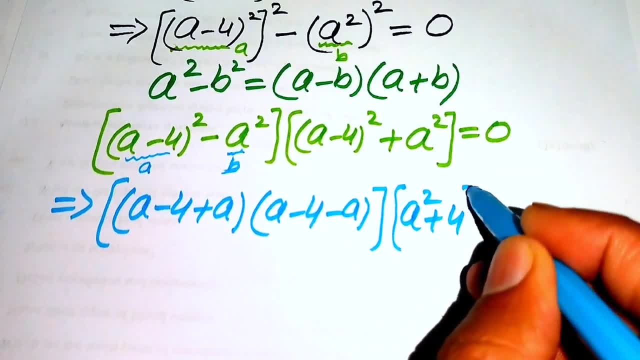 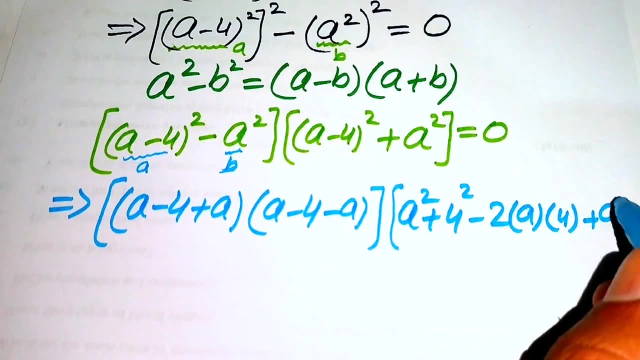 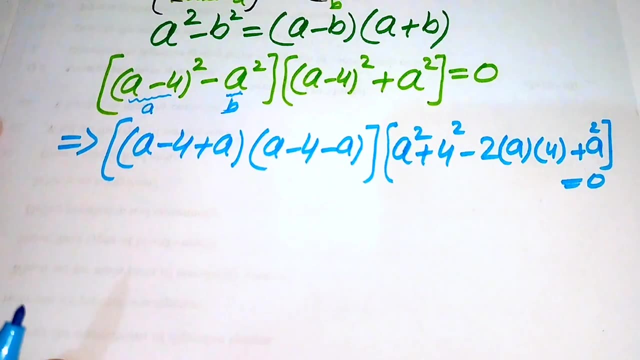 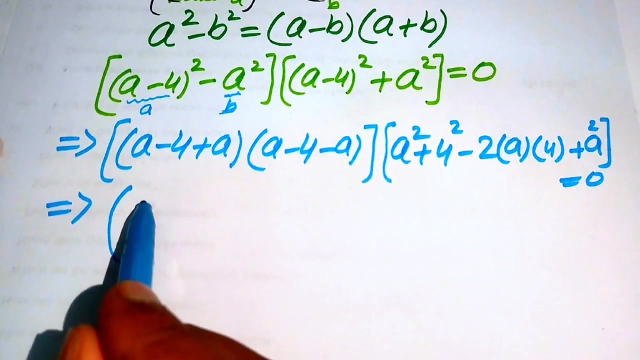 as a square plus b, square minus, 2 times of a into b and plus a square, and this whole equation equals to 0. so in the next step we just simplify the terms and here we obtain: a plus a becomes 2a minus 4, and here we cancel these terms and we 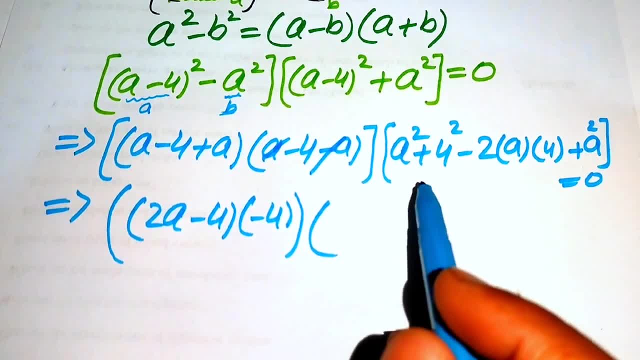 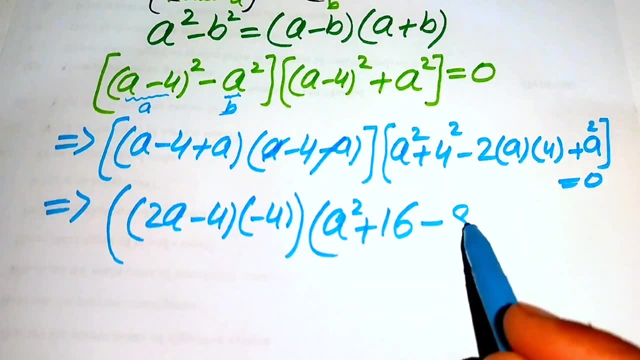 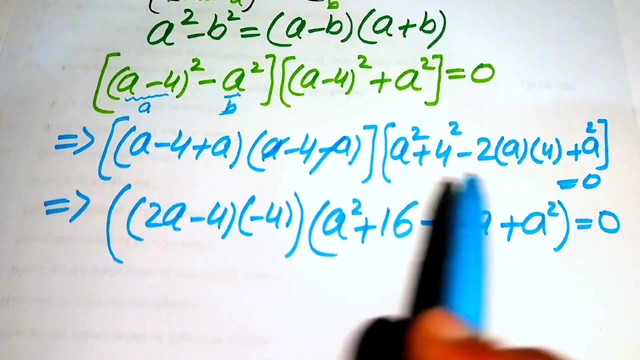 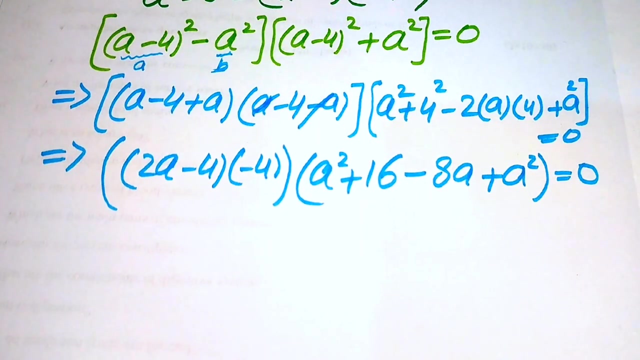 obtain minus 4, and here we obtain a square, and plus 4 square is 16. minus 2 times of 4 is 8a plus this is a square, and this whole equation equals to 0. so now here we have two cases. so our first case is we write: this equation equals to 0 and it will be. 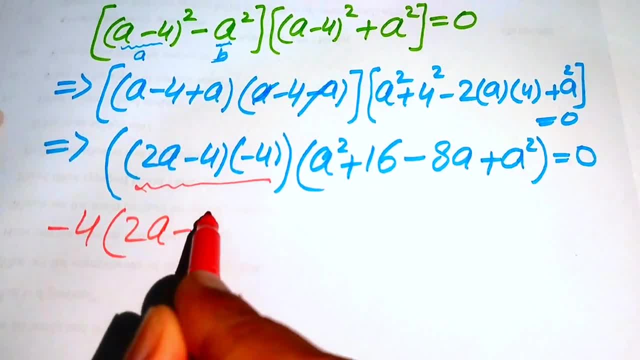 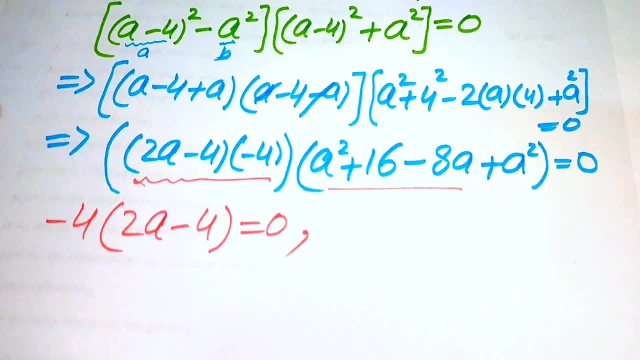 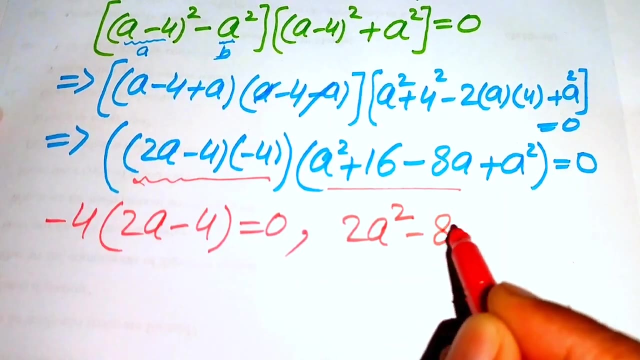 written as minus 4 times of 2a. minus 4, equal to 0. and the second case is we write this whole expression equals to 0. so here, first we add a square plus a square, it will becomes 2 times of a square and we have minus 8a and plus 16. 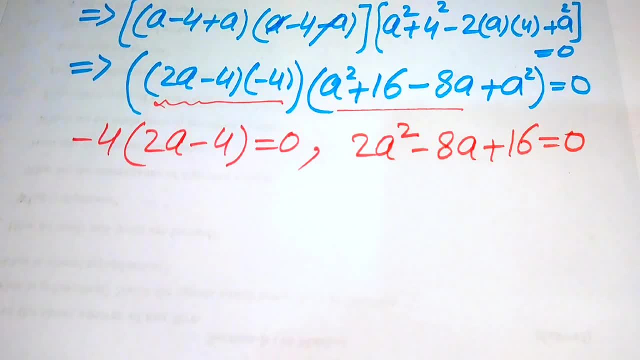 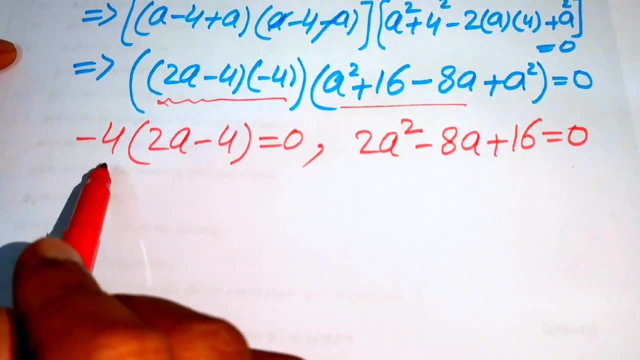 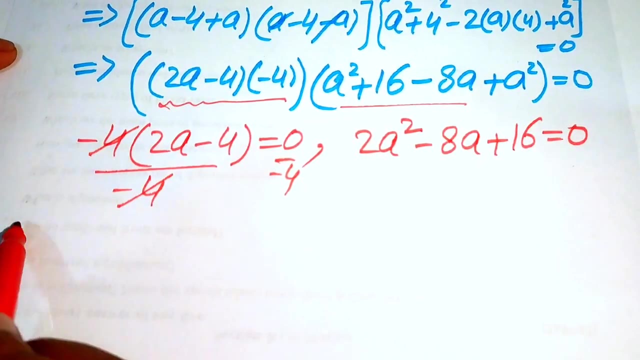 equals to 0. so now we find the value of a from this case. so in this case we move this minus 4 to the right hand side, or we divide both of the sides by minus 4 and you see that this minus 4 is cancelled out by this minus 4 and we obtain 2a minus 4 equals to 0. 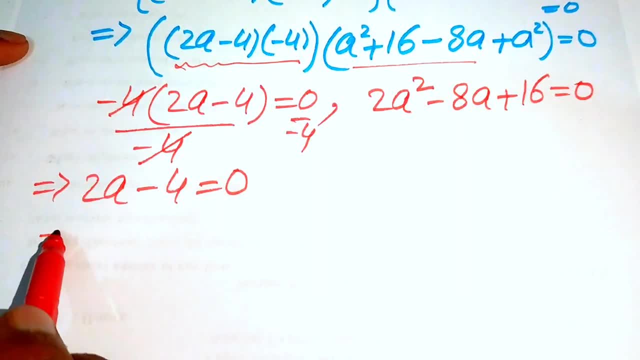 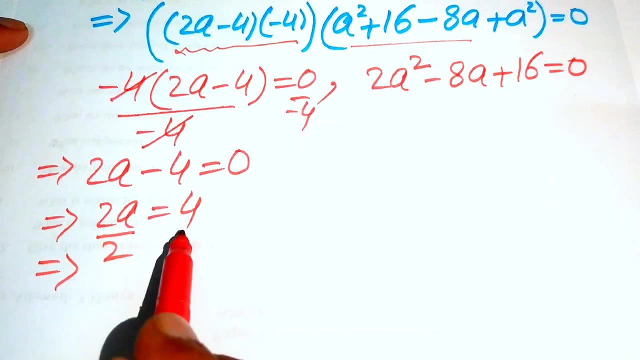 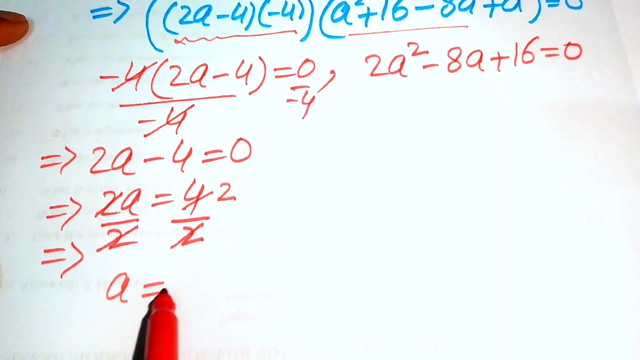 and now, in the next step, we move this minus 4 to the right hand side and it will becomes 2a, equals to 4. and here we divide both of the sides by 2 and you see that this 2 is cancelled by this 2, and this 2 times of 2 is 4 and we get a equals to 2. and now, in the next step, 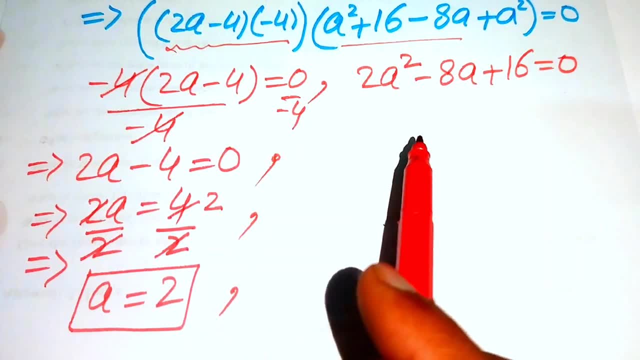 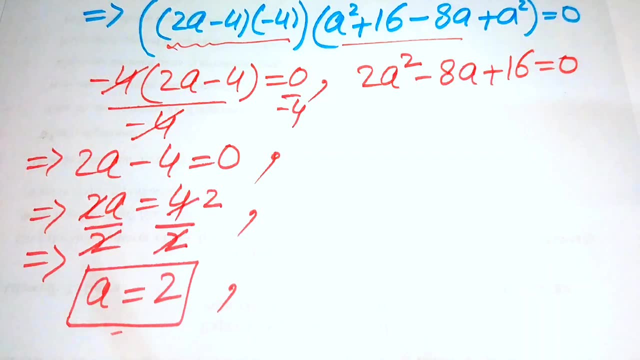 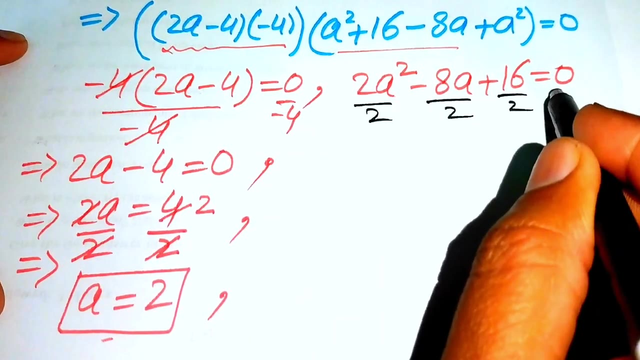 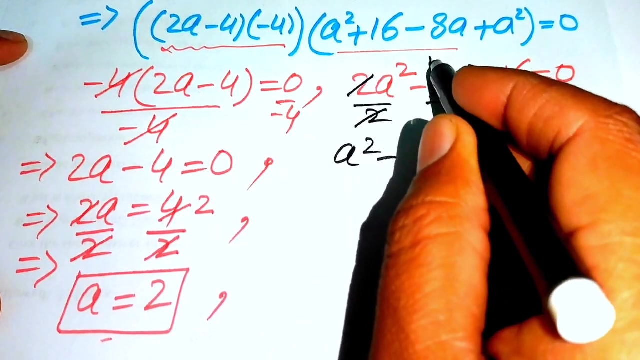 we move towards this quadratic equation because in the first case we get the value of a and now we can simplify the second case, and in second case, first we divide each expression by 2, so in this way, and here you see that this 2 is cancelled by this 2 and we obtain a square minus this 2, 4 x 8, and it is: 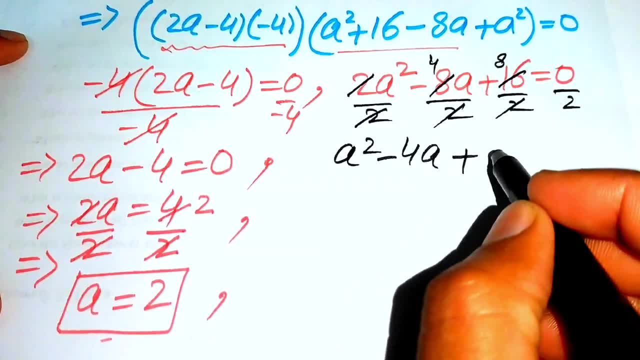 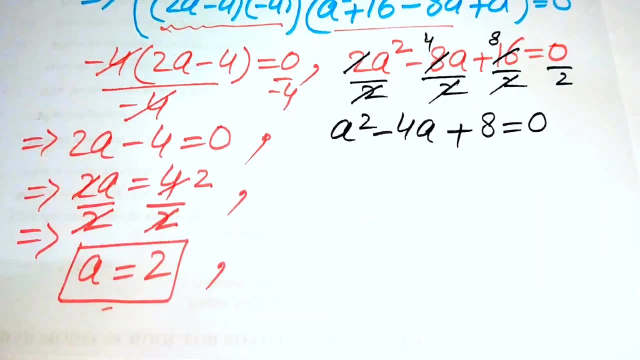 minus 4 times of a and plus 2, 8 x 16, and 0 over 2 becomes 0. so in the next step we can easily make the factors of this equation, or in other words, we will use the quadratic formula. so now, here we use the quadratic. 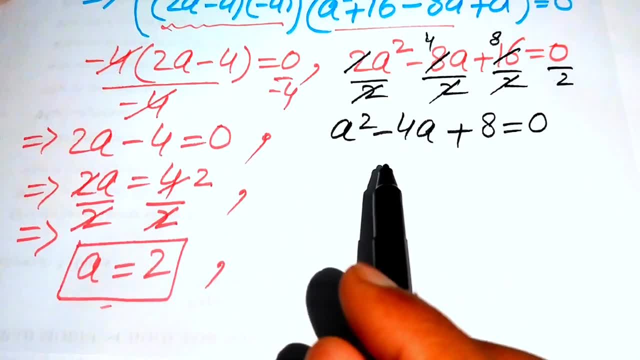 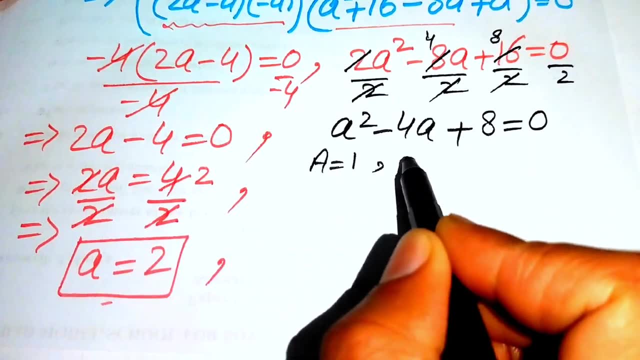 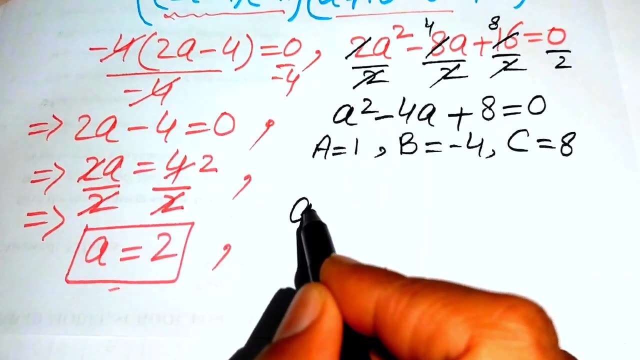 formula. so in order to use the quadratic formula here, we need the exponents of this equation. so the exponents of this equation are: a equals to 1, b equals to minus 4 and c equals to 8, and our quadratic formula will be looks like in: 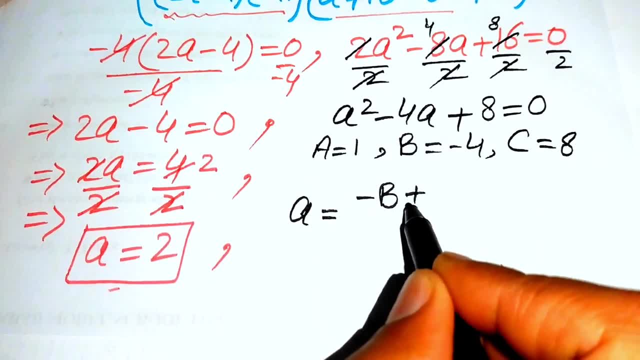 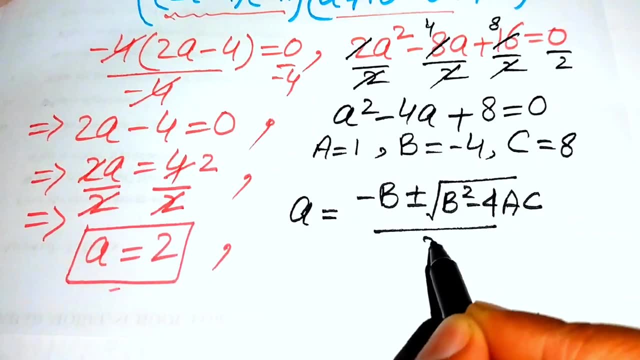 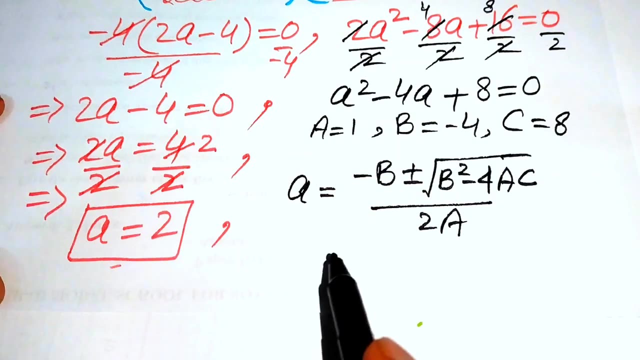 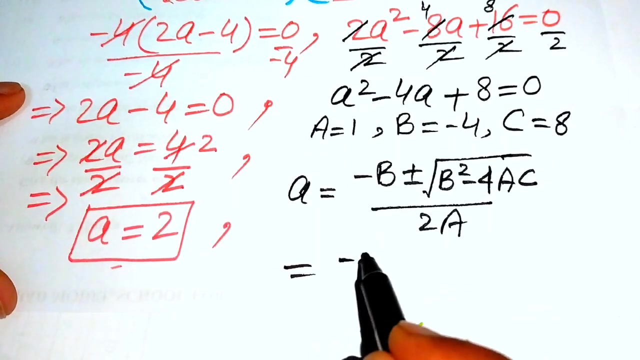 this form, a equals to minus b plus minus square root of b squared minus 4 times of a, c divided by 2 times of a. and now we can substitute the values of ab and c in this quadratic formula. so the value of b is minus 4 and it will be written as minus times of minus 4. 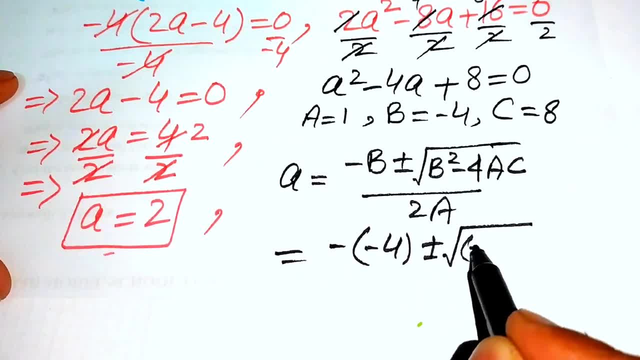 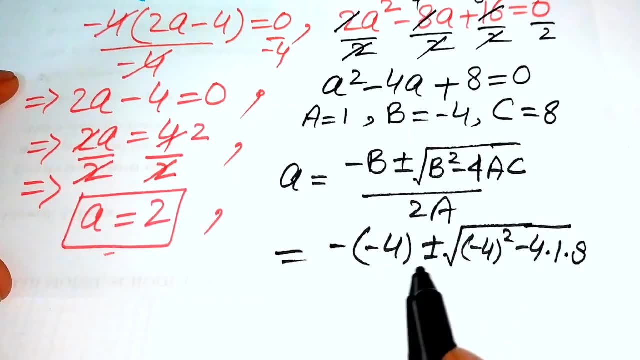 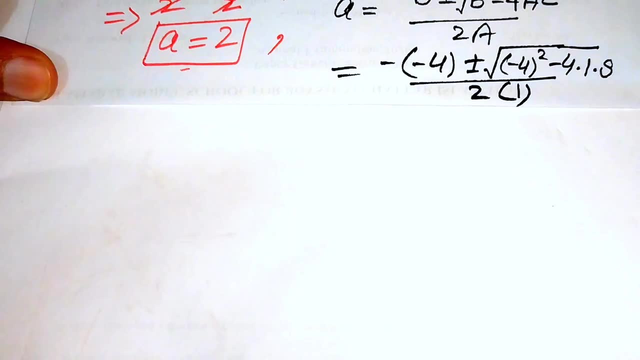 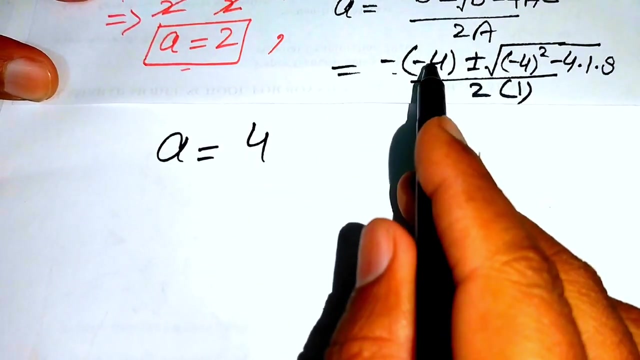 plus minus square root of b square. so our b is minus 4 square, minus 4 times of b. squared a into c, divided by 2 times of a, and our a is 1. and now, in the next step, we will simplify all these terms and we write it as: a equals to 4, because this is minus, times of minus becomes plus. 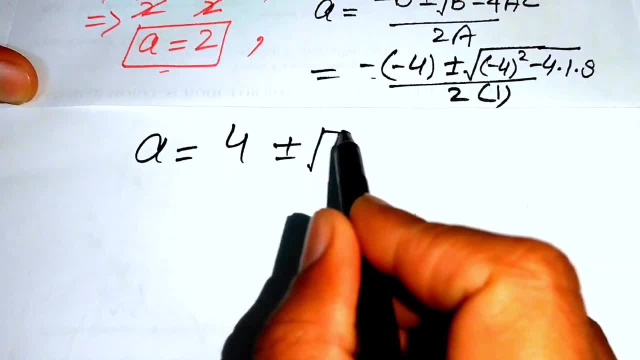 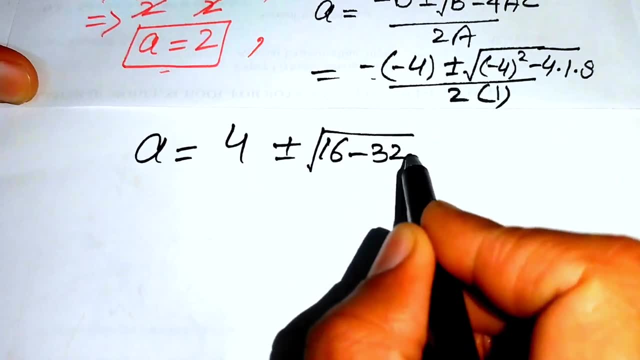 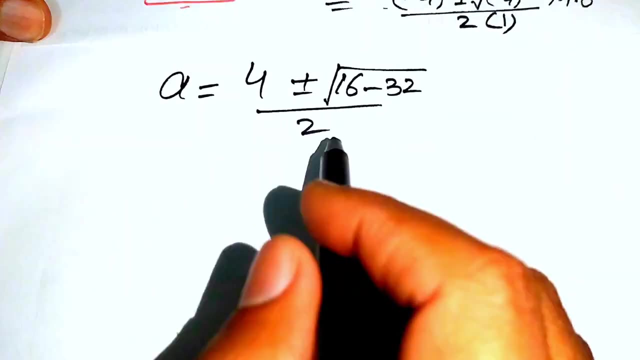 4 and plus minus square root of minus 4 square is 16, and a 4 times of 8 is 32, divided by 2 times of 1 is 2, and now here we simplify this equation and we have a equals to 4 plus minus 16, minus 32. 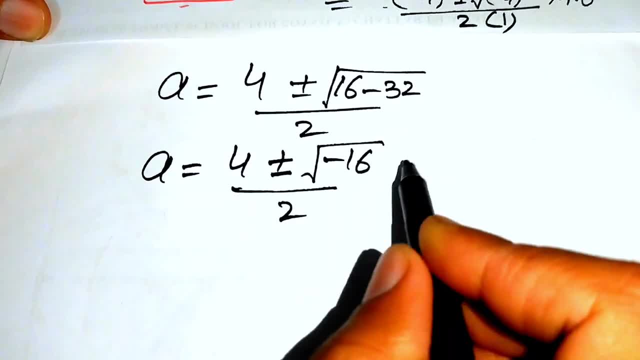 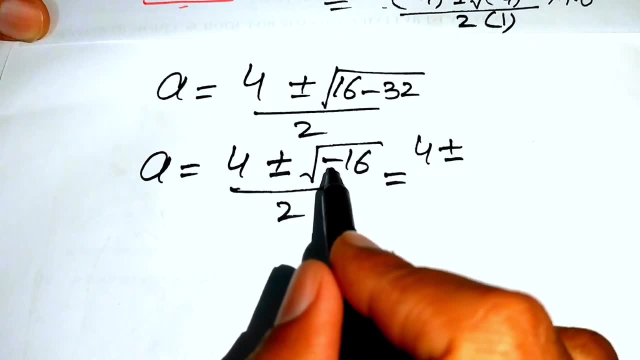 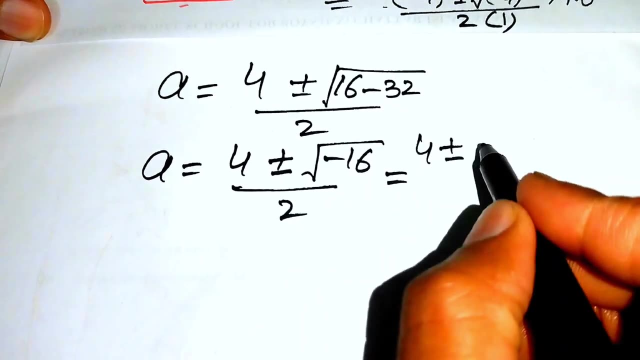 becomes minus 16 square root divided by 2. and here you see that we have 4, 14 plus minus. so here you see that the negative sign becomes inside the square root. so it will be equals to iota, and we know that the square root of 16 is 4 times of iota divided by 2. 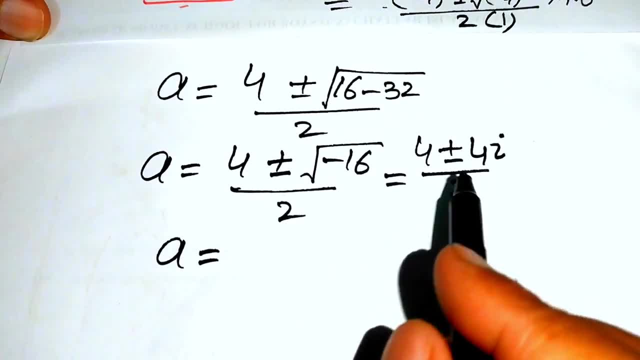 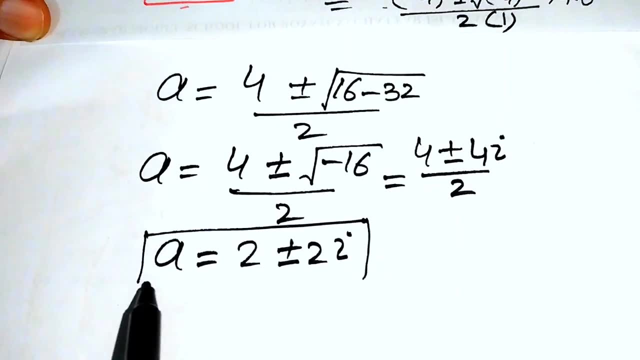 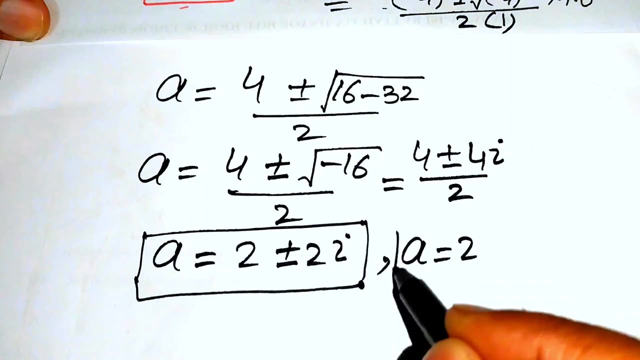 and we have a equals to. so we separate these two terms and we get 2 plus minus 2 times of iota. so these are the other two complex roots of the given equation- and it's one real root- are a equals to 2. so this is the our final answer of this question and thank you so much for. 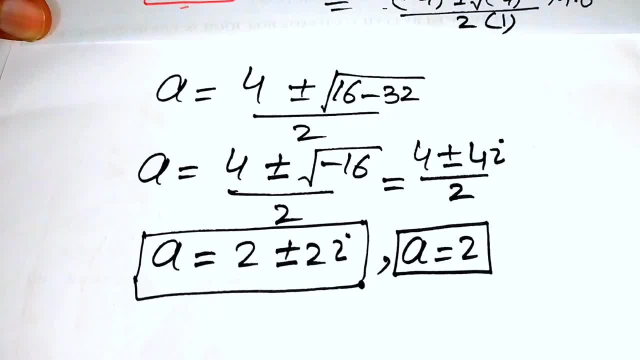 watching this video. please subscribe to my channel for more exciting videos.